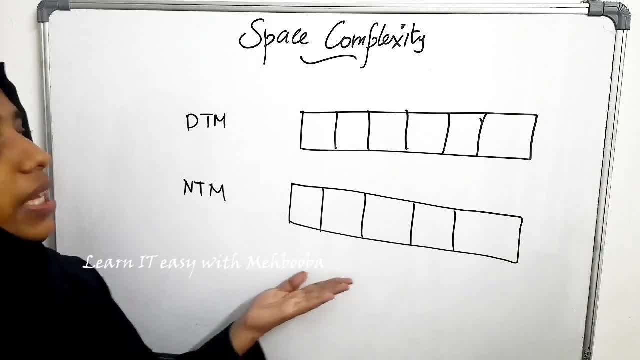 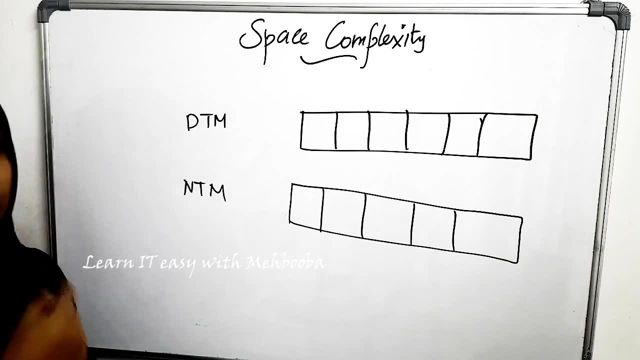 computation, and that actually attributes to the space complexity of space complexity. we are defining space complexities like that. you know that turing machines are hypothetical models of modern day computers, and hence this definition really makes sense. now we have different measures and definitions here, so we will see them one by one. 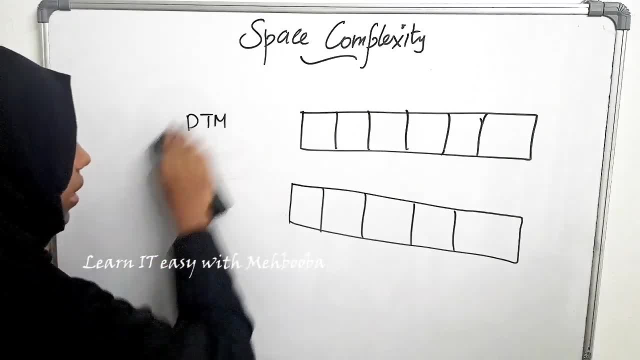 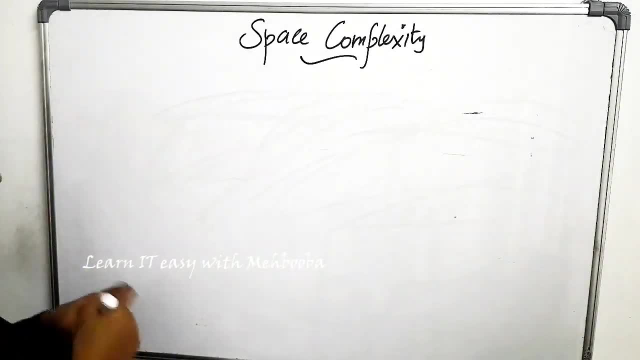 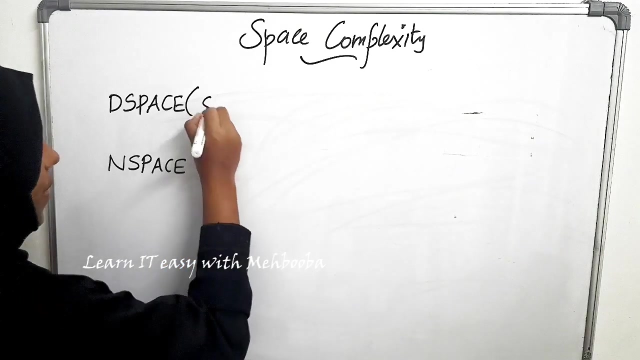 so the two main categories, or two main. your divisions is like d-space and n-space, d-space or simply space and n-space. ok, in some textbook it will be simply space, d-space or n-space. d-space of s of n, where s of n is the time, complex space complexity. and space of s of n, where s of n has. 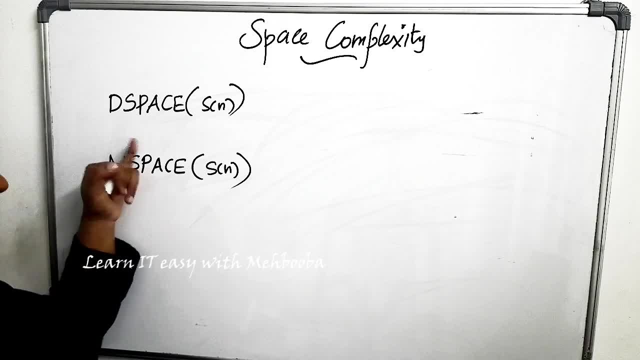 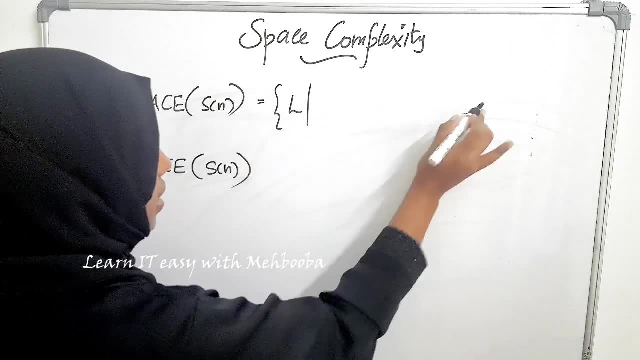 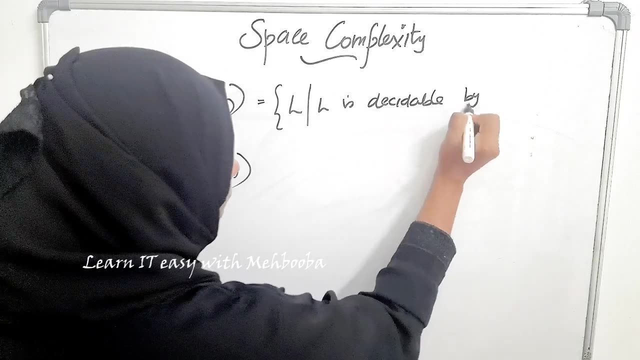 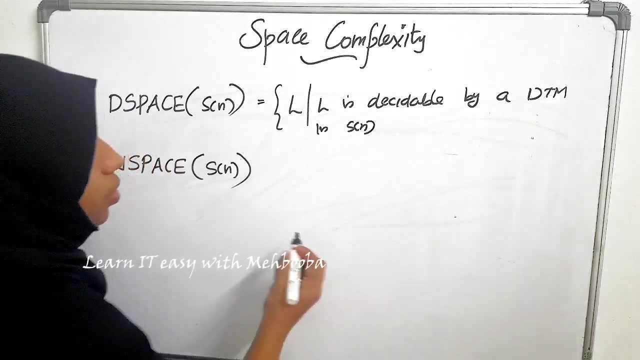 the time complexity of n as the space complexity. So I mean now I will give you the definition So d space, of s of n, as the set of all the languages such that L is decidable by a deterministic Turing machine in s of n space. Okay, So this is the set of all the languages which 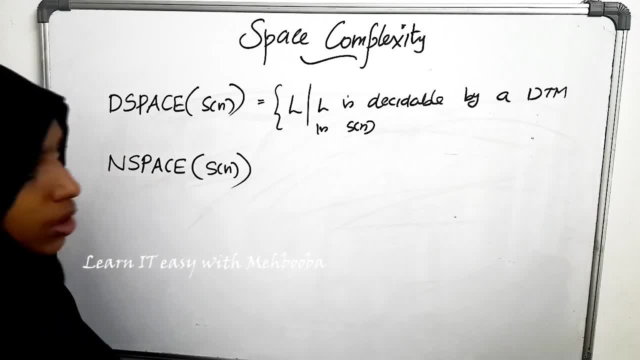 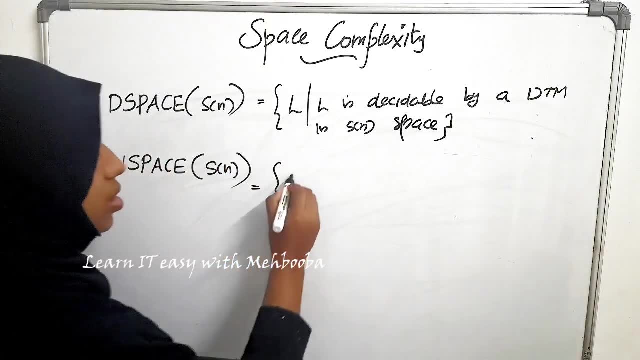 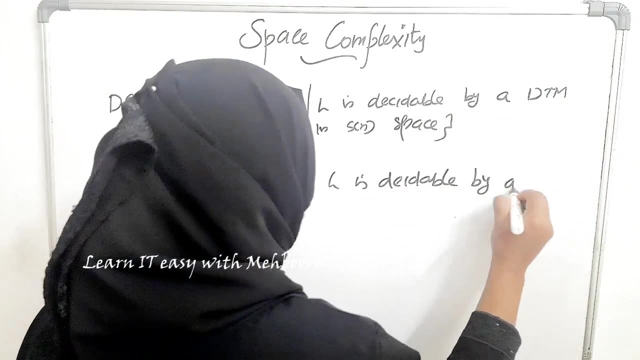 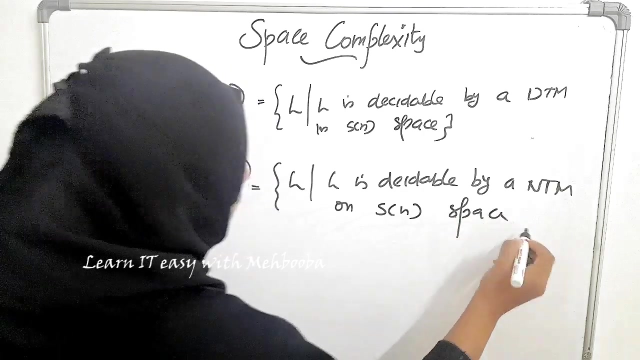 are decidable by a deterministic Turing machine in s of n space. So, similarly, as you can imagine correctly, n space is the set of languages where L is decidable by a non-deterministic Turing machine on s of n space. Okay, So yeah, simply speaking d space is the space. 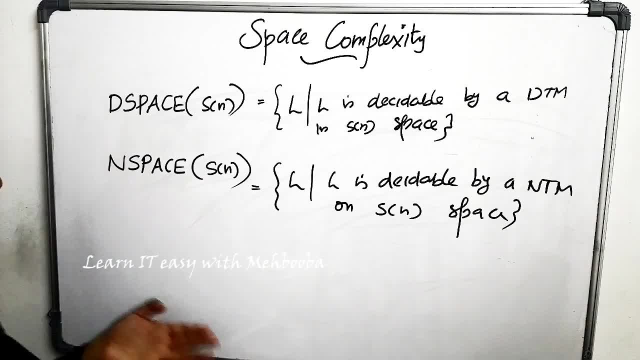 taken by a space. So d space is used up by a deterministic Turing machine and n space is the space used up by a non-deterministic Turing machine. Now, just like we have complexity classes, P and N P in time complexity, we have P space and N P space analogous to that P space, and 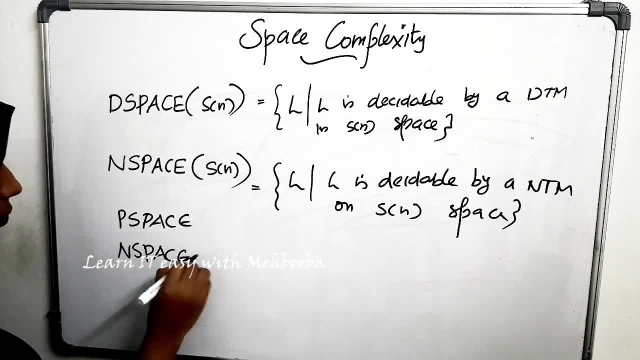 N space analogous to P and N P complexity classes in terms of, in case of Turing machine. So this is the set of all the languages which are decidable by a set of all the languages. So P space and N space are the other complexity classes here. So P space is actually the 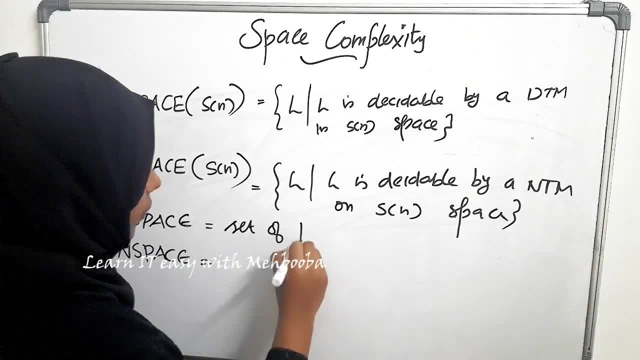 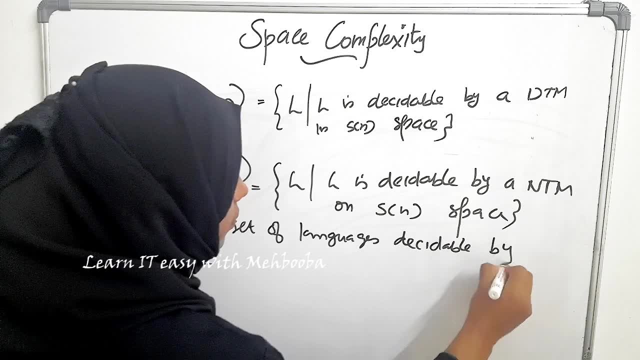 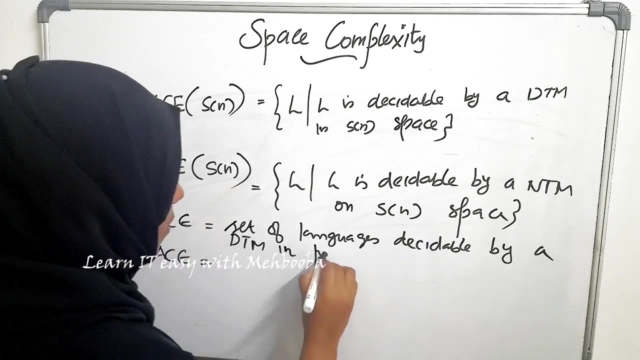 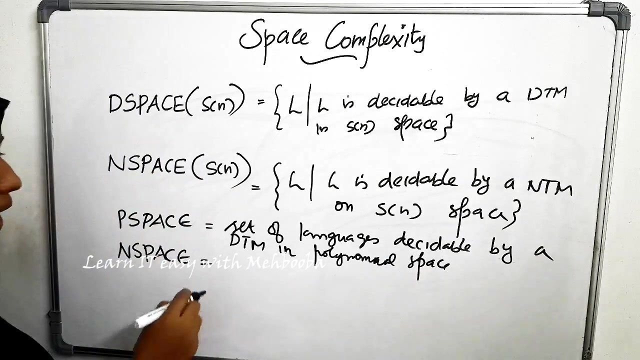 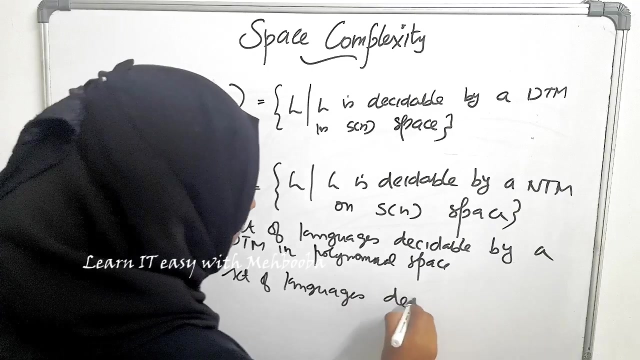 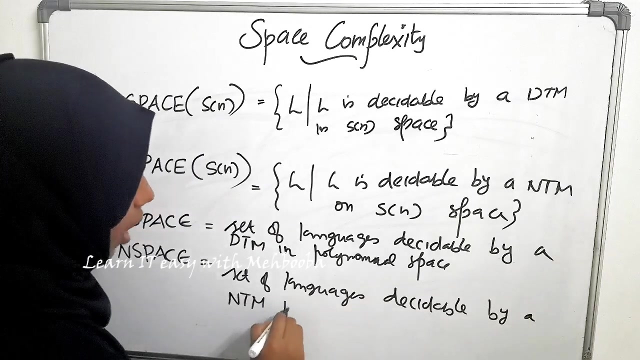 set of languages decidable by a deterministic Turing machine in polynomial space. that is the polynomial space here. So similarly, n space is the set of languages decidable by a non-deterministic Turing machine, NTM, in polynomial space itself. See, you may get. 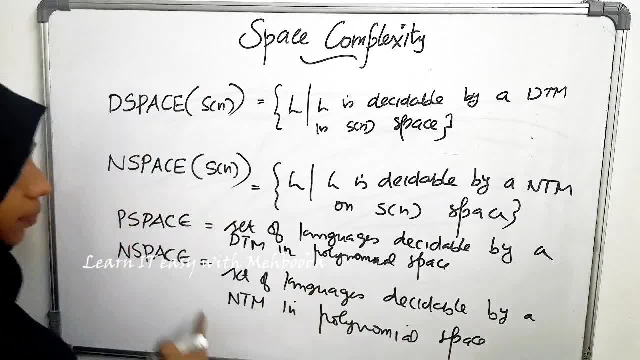 confused why it is polynomial space in both the cases. that is why it is still polynomial or n space. So this is true for n space and n space, as we are working on a non-deterministic Turing machine. See, we will see a theorem in the next video named as Savage theorem. 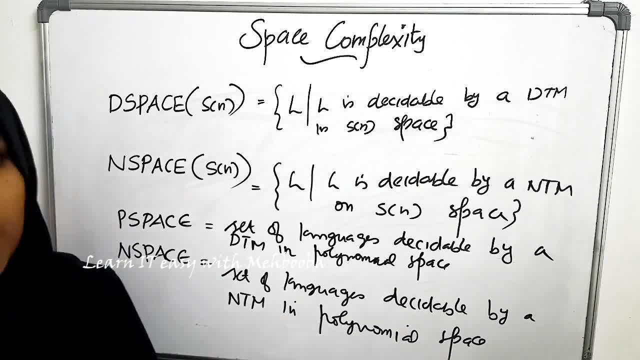 which shows that P space is equal to n space. So then you will understand how come the space complexity of a deterministic Turing machine and Non-deterministic Turing machine are both polynomial in nature. We will see that in the next video when we discuss the 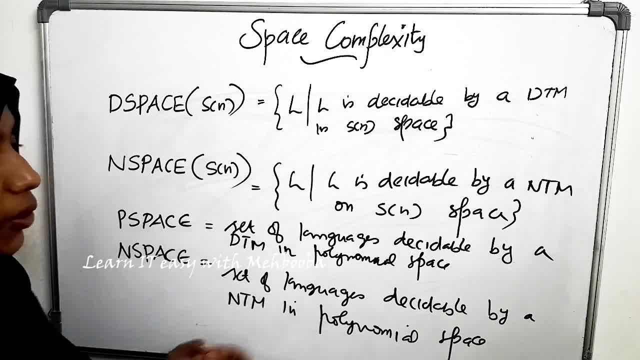 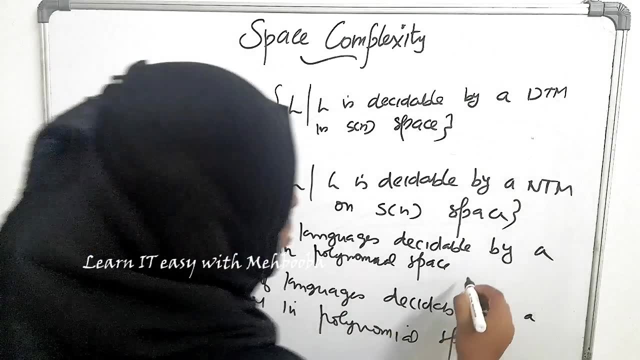 Savage theorem. So for the time being, just understand that P space is a set of languages, is decidable by a deterministic Turing machine in polynomial space, and n-space is a set of languages decidable by NTM in polynomial space itself. You can also write it as the set of: 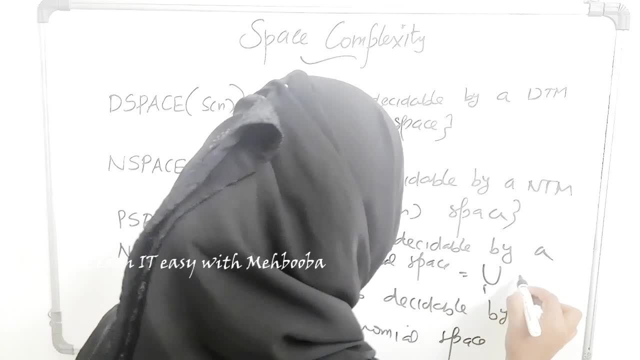 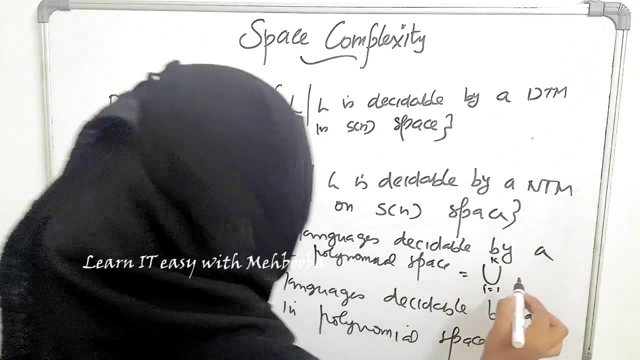 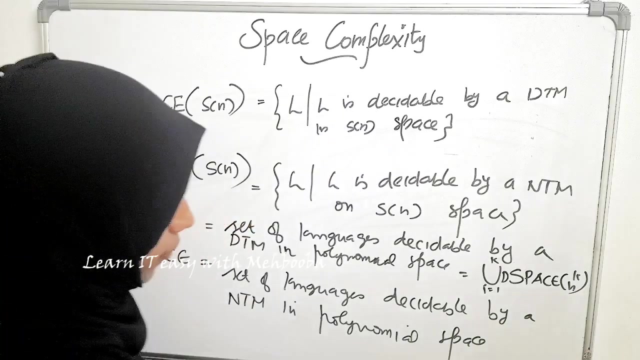 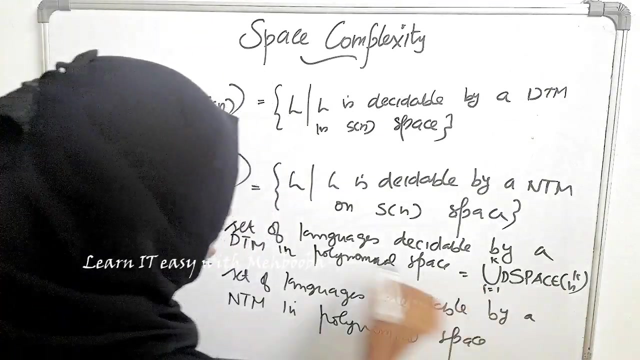 all the languages for O line, Union of all such languages which take just d-space. d-space is the time complexity for a deterministic Turing machine. I mean set of all languages which take space by a deterministic Turing machine, but it is in polynomial time. This 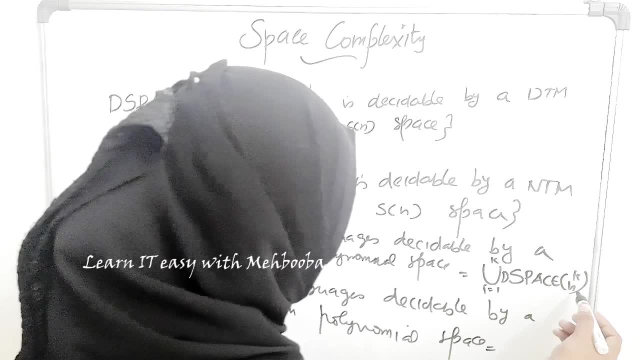 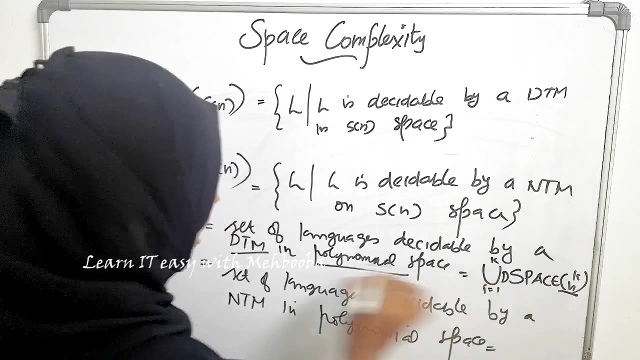 is polynomial time because n raised to k, Where n raised to k is a polynomial, d-space indicates that it is a deterministic Turing machine. n raised to k indicates that it is a polynomial time. This union indicates that it is a set of languages, So similarly it 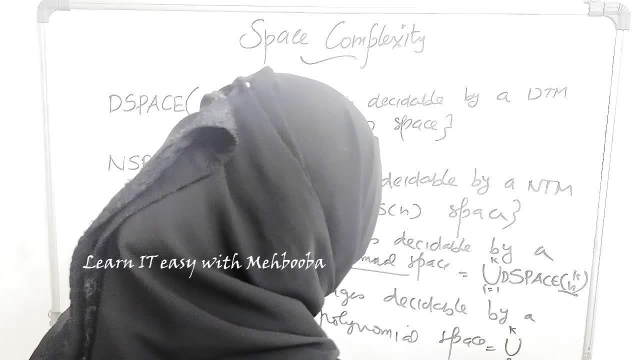 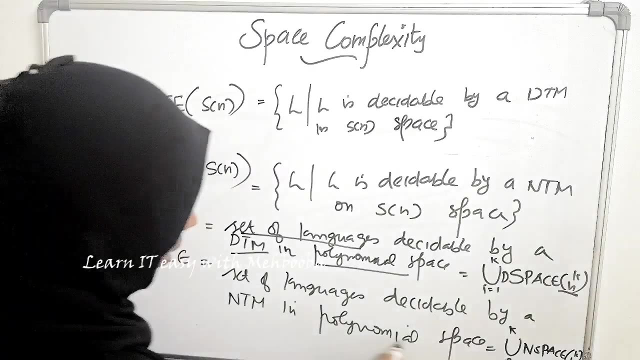 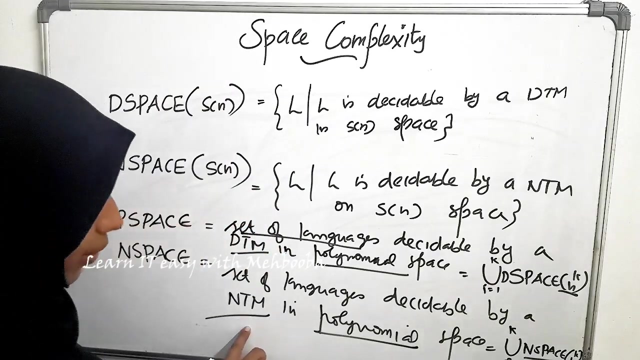 is union over I. i is equal to 1 to k. n-space of n raised to k, n raised to k indicates that it is taking a polynomial space. n-space indicates that it refers to the space complexity of a non-deterministic Turing machine. and this union indicates that. 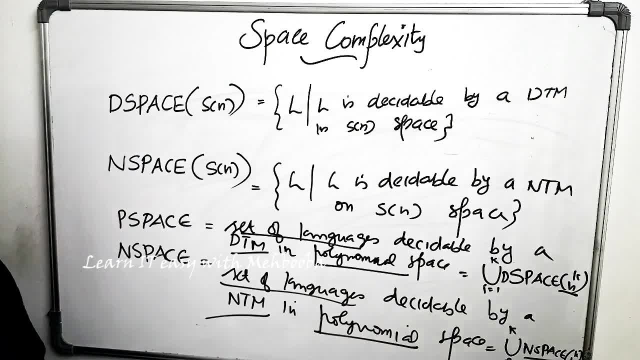 it is a set of languages, So this is how we define this. This is d-space and n-space. This simply refers to the space taken by deterministic Turing machines. This refers to the space taken by deterministic Turing machines, by a non-deterministic turing machine. p space is analogous to the complexity classes- complexity. 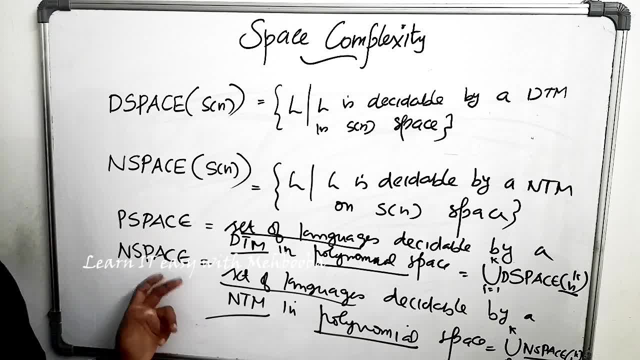 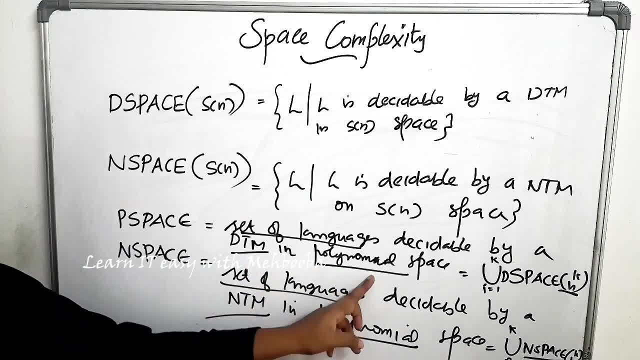 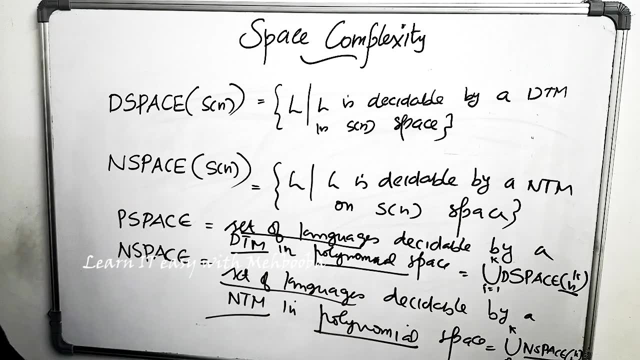 class p in time complexity, and space is analogous to the complexity class n, n p in time complexity. p, space is a set of languages desirable by dtm in polynomial time, and space is a set of languages desirable by an ntm in uh polynomial space itself. and you know what exactly is decidability if you. 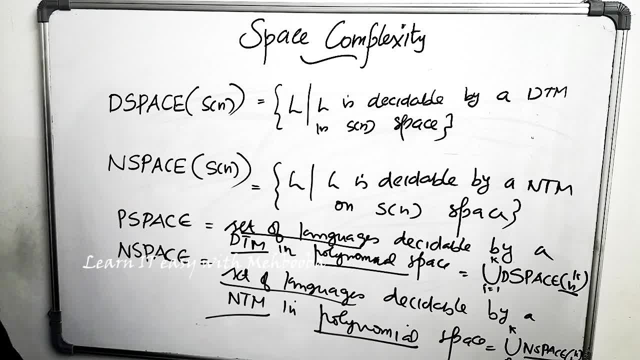 don't know, please to watch the previous video on decidability. okay, i mean. decidability means i mean the turing machine can uh, give a proper, i mean decide the language, that is, given a particular input, whether the turing machine can correctly say that i mean, uh, the machine will stop on. 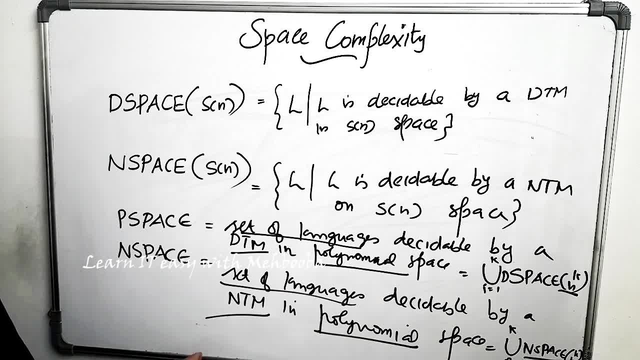 every input, saying either yes or no, or by either accepting it or rejecting it. okay, so these are the basic notions in case of uh, time, complex, space, complexity, you. we also have uh classes, uh which uh, which are l and n, so l means uh logarithmic, uh complexity class. 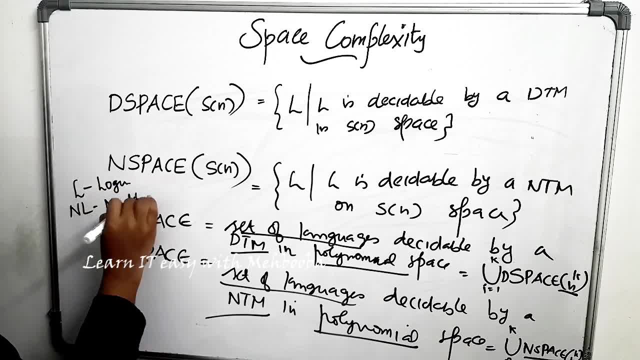 logarithmic. this is a non-deterministic logarithmic complexity class. non-deterministic logarithmic complexity class. we will see these two classes in one of our next videos, after savage theorem, probably so. l means the algorithms which take logarithmic space. the class only includes uh. 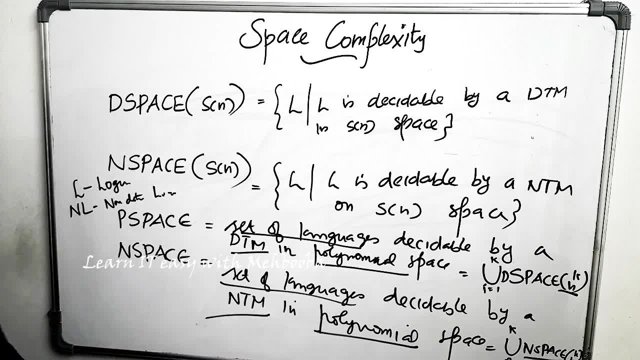 computer computational problems which take, um, yeah, logarithmic space. and uh, nl includes, uh, the uh computational problems which is solved by a non-deterministic turing machine which take local space. so we will see these two in detail in one of our upcoming videos. so, uh, for the time being. 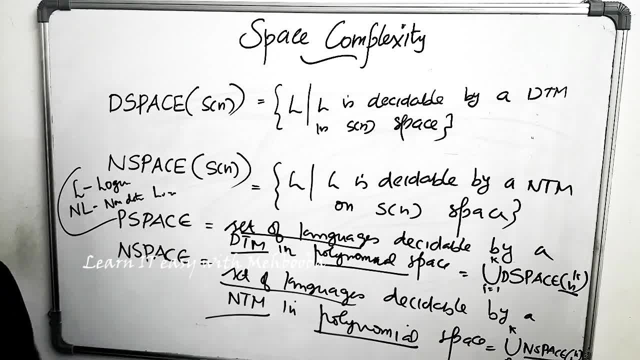 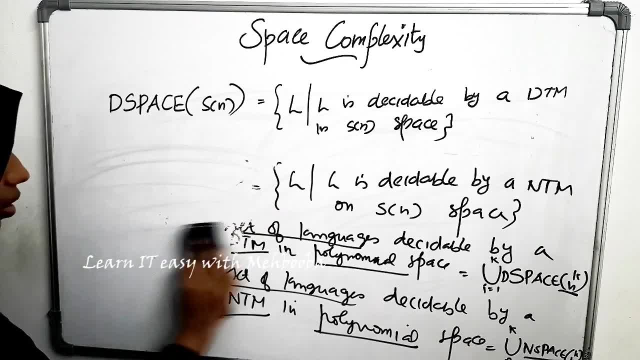 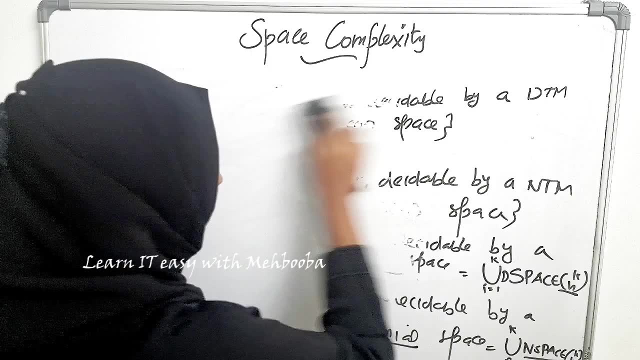 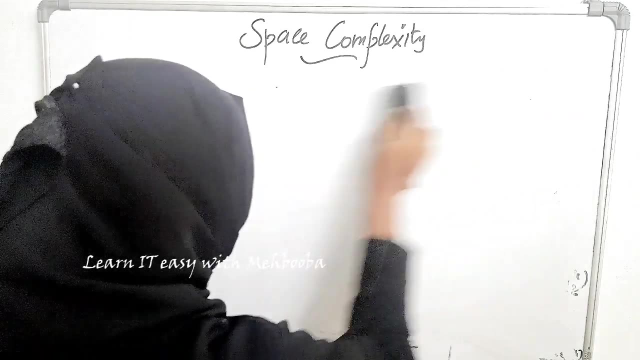 we will be discussing, we will be restricting our discussion on these complexity classes. so now, uh, we will um just uh see the very the side problem which we were using all this while to uh as the basis of proving everything, to uh the class np complete in case of time, complexity, and we will, as an example here, we will just analyze. 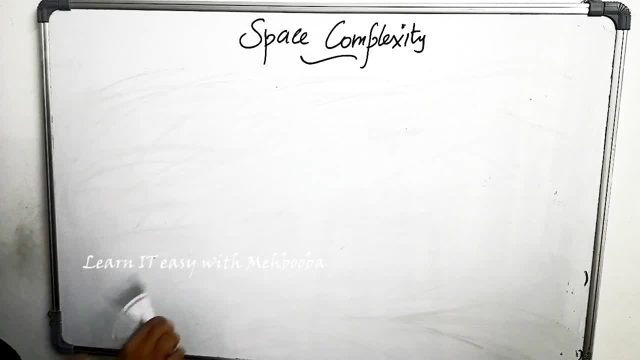 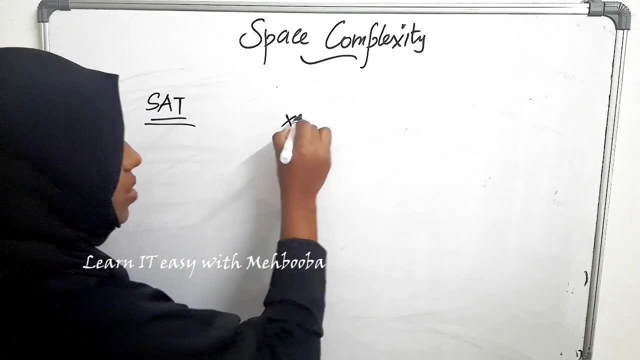 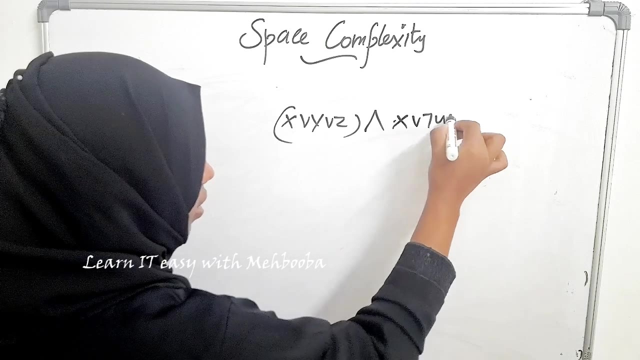 uh, the space complexity of the start problem. so hope you're remembering that start problem deals with the satisfiability of formulas. that is, given a boolean formula like x or y or z and um, x or negation, why? or negation, is it formulas like design, whether these formulas are. 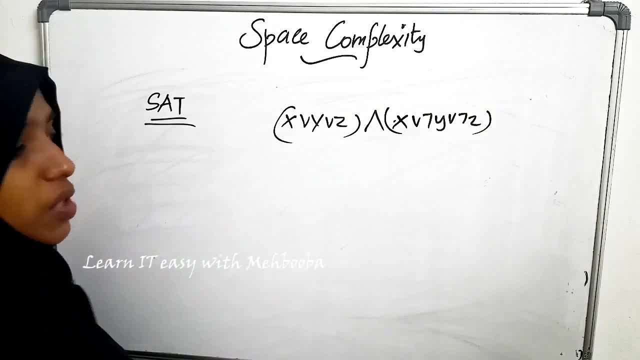 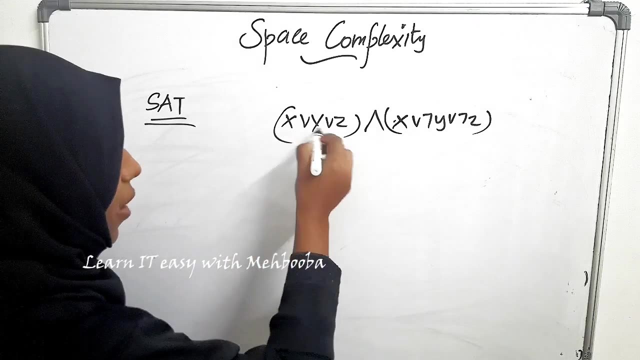 satisfiable or not. so uh, start problems deals with formulas like this. so, and if at least one truth assignment to this variables can lead to a one in the output, the formula is satisfiable. otherwise it is not satisfiable. we have discussed it, so here we have several. 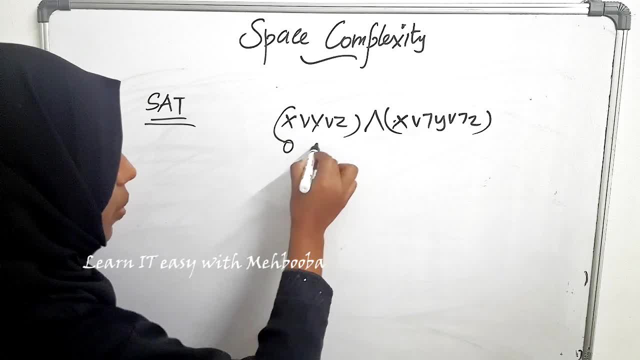 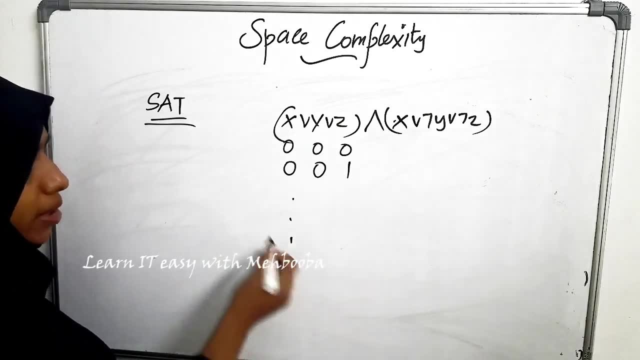 different truth assignments. for example, you can give 0 to x, 0 to y and 0 to fps to z, 0 to x, 0 to y and 1 to z, and it goes on. You will get 8 different truth assignments. 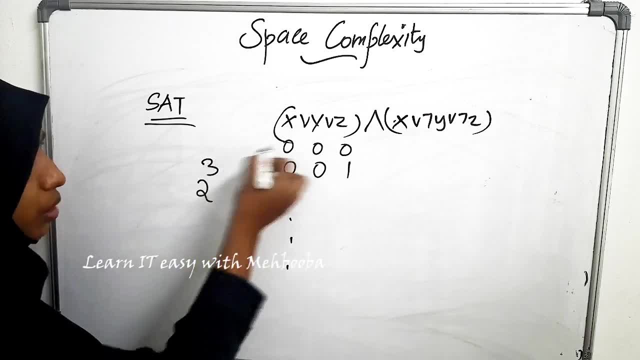 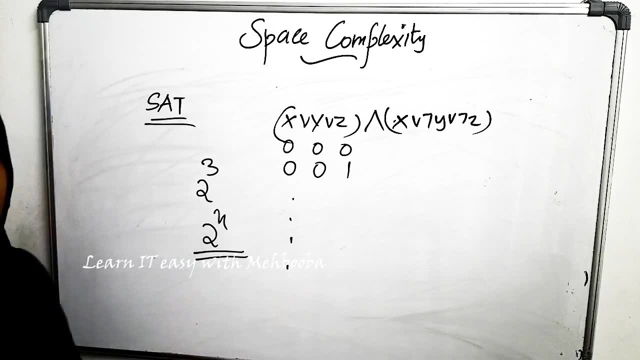 because there are 3 variables and 2 raised to 3 truth assignments are possible and for n variables we have 2 raised to n truth assignments and you know that this is exponential. So SAR problem is taking exponential time and it was NP and NP complete. but we will see. 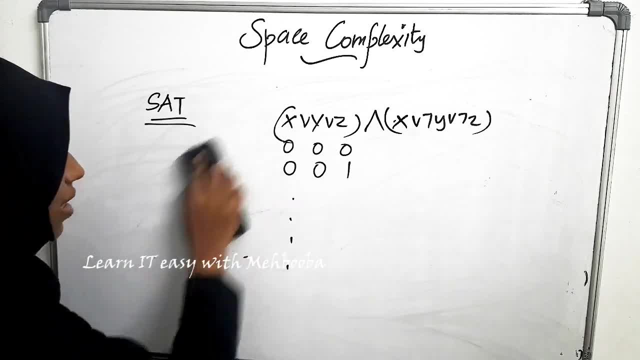 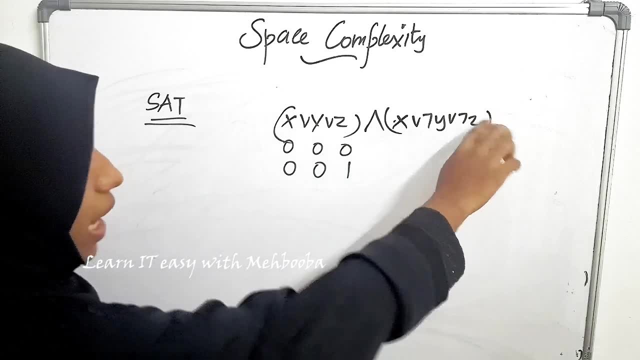 how does SAR performs in terms of space complexity See? if you want to give x 0, y 0 and z 0 and check the acceptability or satisfiability of this formula, you can do that, For example: 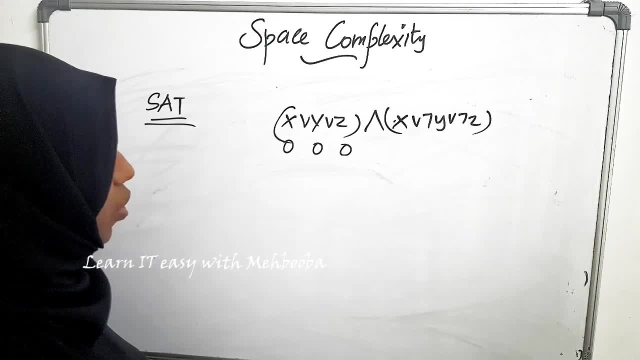 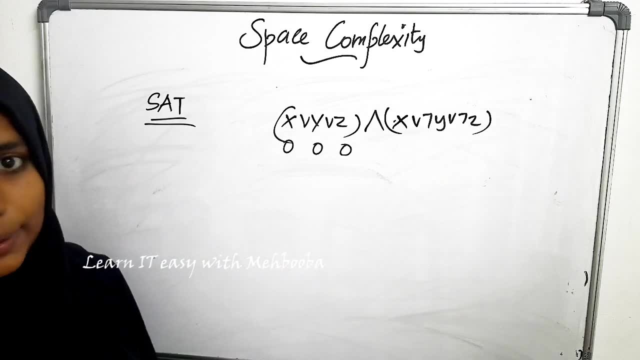 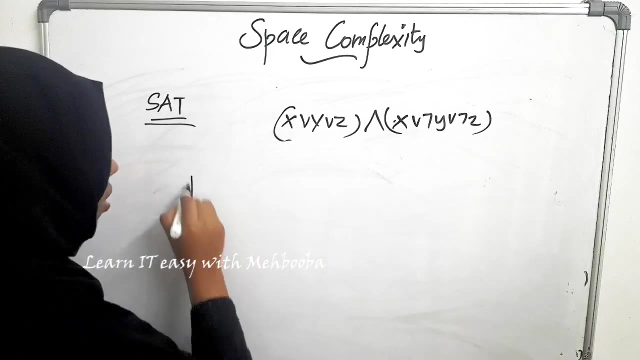 you can give x as 0, y as 0, z as 0 and these 3 assignments can be stored and you can get the value of this formula. Now, if you want to try with another complex combination, that is, 1, 0, and if you want to check this with 0, 0, 0, you can save that. 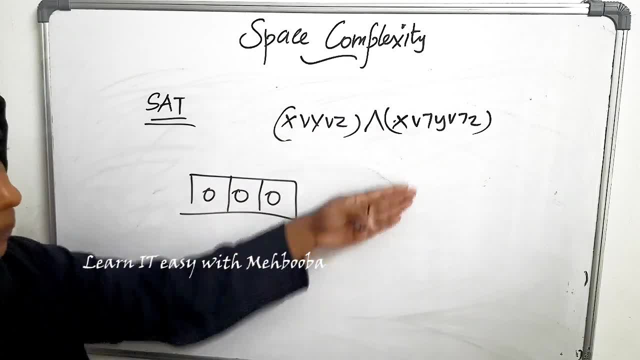 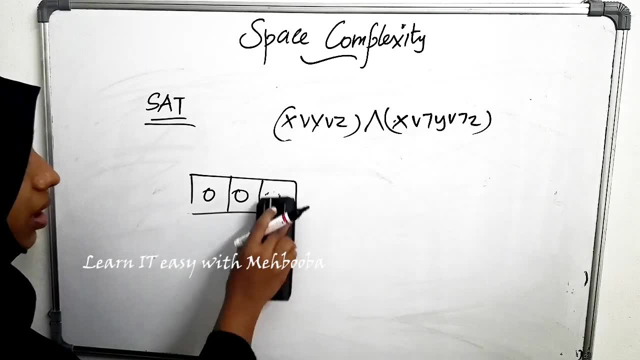 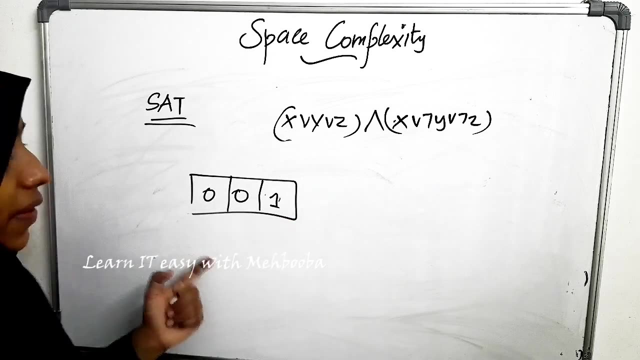 assignment in a tape and verify the truth value of this formula. Now, if this is not working and in the worst case, if you want to try with another configuration that is 0 for x, 0 for y but 1 for z, you can delete or remove the previous assignment stored in. 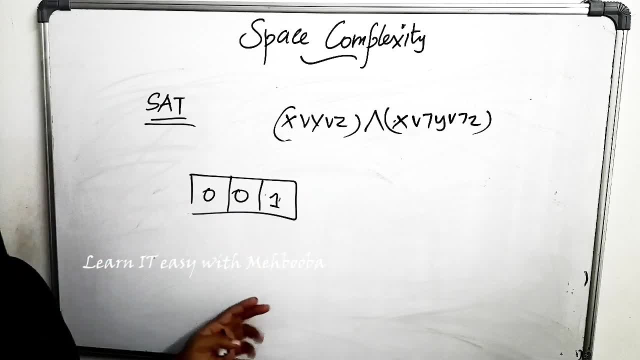 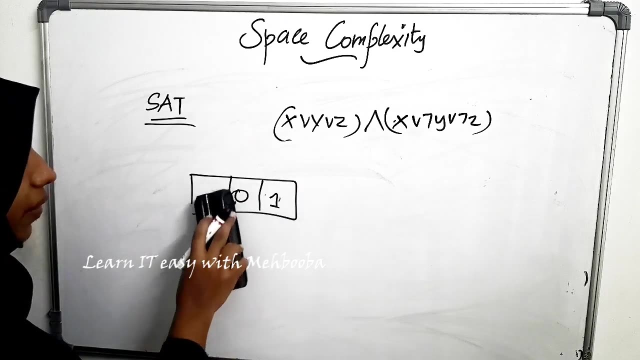 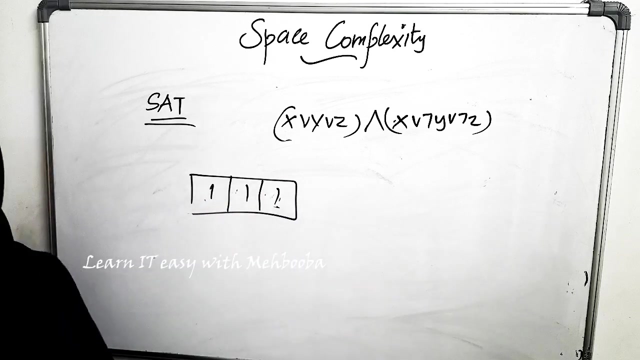 the tape and the same tape cells can be reused. So the same tape cells can be reused again. for all the computations, all the different assignments, The same tape cells can be reused. For example, if you want to try with giving 1, 2, x, 1, 2, y and 1, 2, z, you can rub this complete assignment and give 1, 1, 1.. So 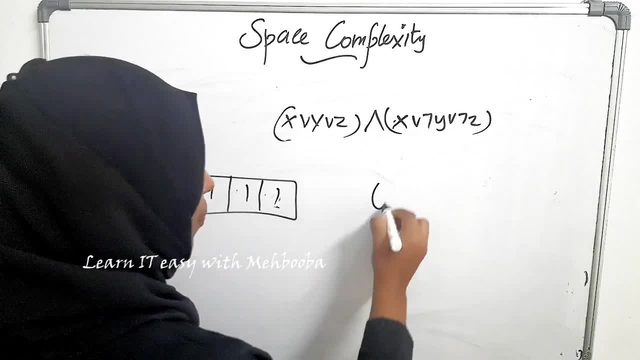 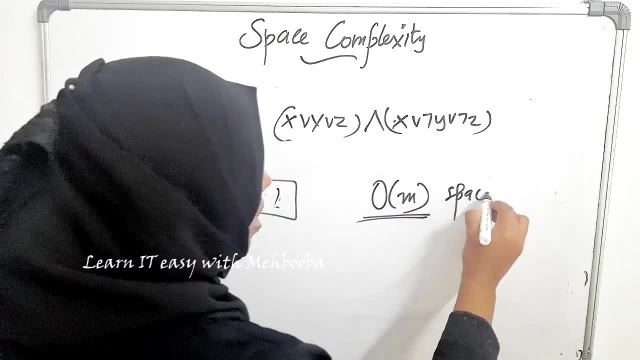 the same tape cells can be reused. So if there are m variables, you just can do this with an order of m space. Now, this is a very big problem, and we are going to talk about another problem, which is called the SART problem. 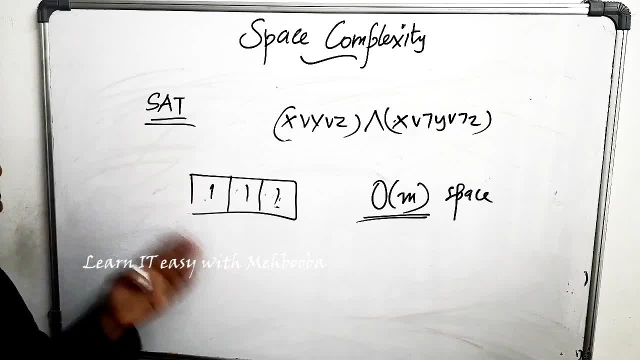 Now we can see that the SART problem is indeed n? p. in case of time complexity It is very linear or it is just taking polynomial space. in case of space complexity, That means even if the space time complexity of an algorithm is really high, the space complexity can be. 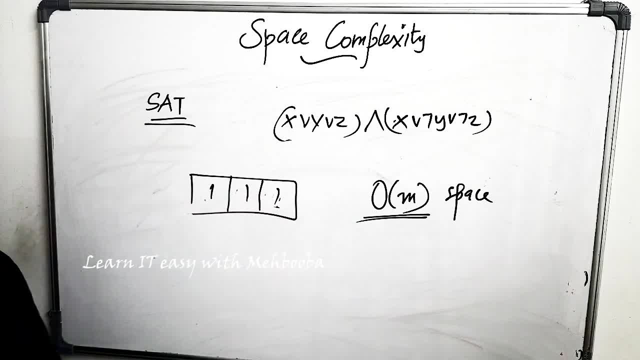 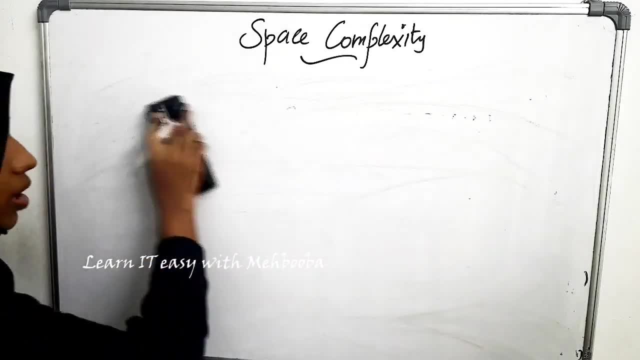 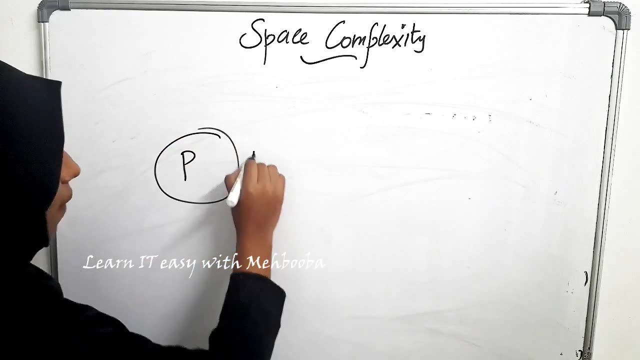 very small. Okay, So that was it. I just wanted to discuss SART, Because we were discussing SART for almost all our examples in time complexity. So this is how SART takes three pleasure table. Okay, now we will see the difference. I mean the relation between the space and time complexity classes. So if I represent it as an inclusion diagram, it will be like this: The class P is the innermost one, then comes class NP and then comes class PSPACE. 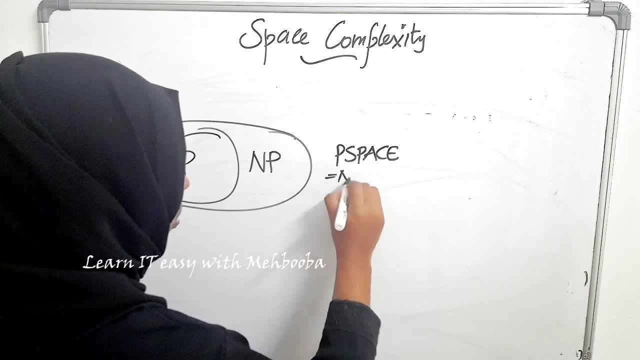 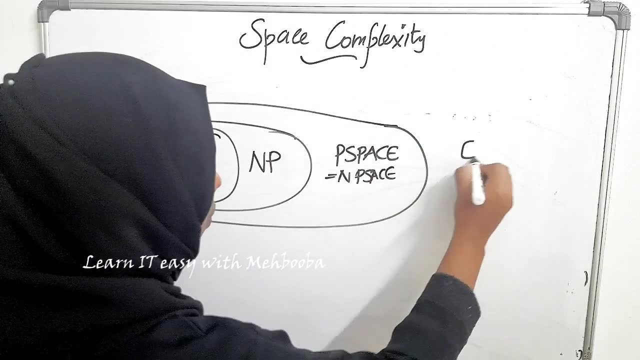 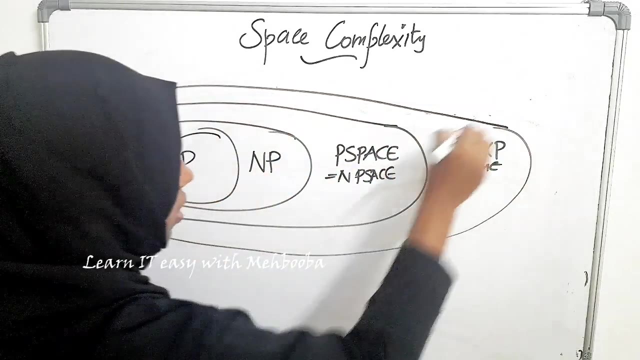 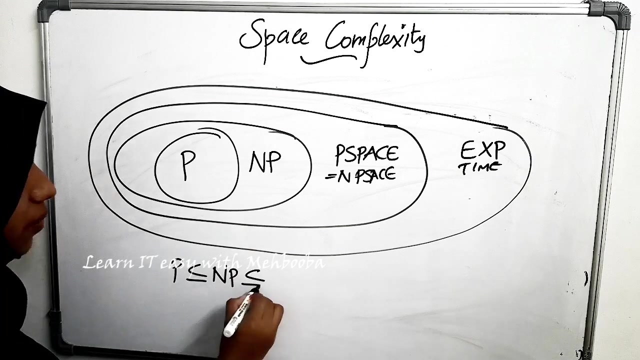 PSPACE is actually equal to NP SPACE, As I have told you earlier. we will use Savage Theorem to prove this, and exponential time is the outermost class. See P is subset of class NP. you know that by this time, isn't it? Now that is subset of class PSPACE, which is actually equal to the class NSPACE. 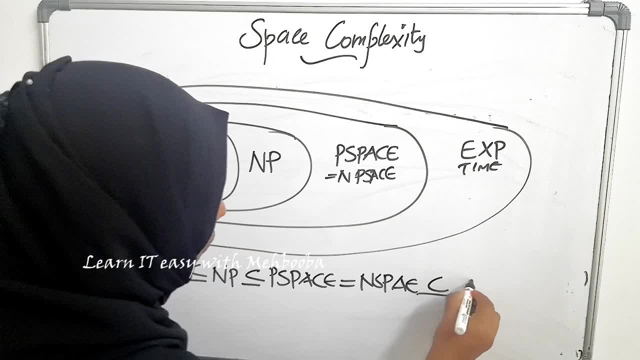 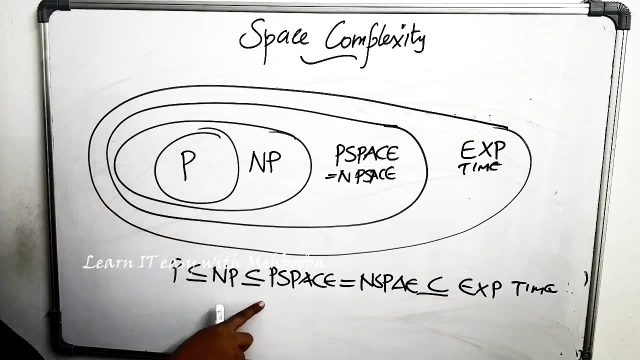 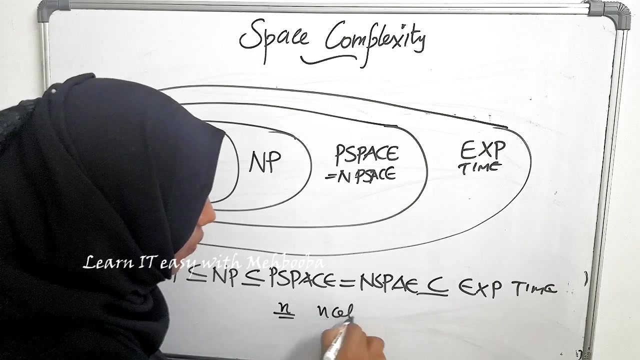 PSPACE is subset of the class exponential time. See, the reason behind P and NP being subset of PSPACE is that while doing any computation, I mean we cannot have more space, or I mean for any. if you are having any computation steps, we will be using N cells of a Turing machine. 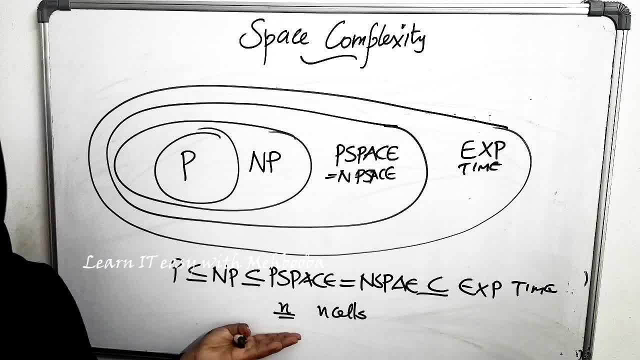 That is, we will be using N cells. So if there are N computation steps, That is no computation which is taking N cells can go more than N cells. So definitely, if you are having N cells, N computation steps, you will be using up N cells. 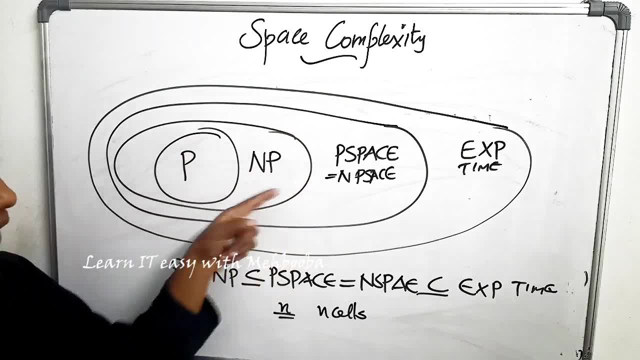 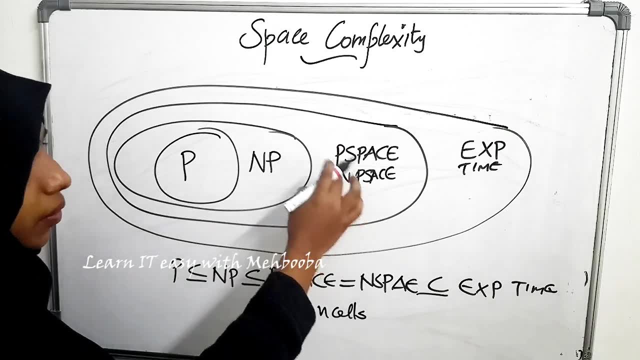 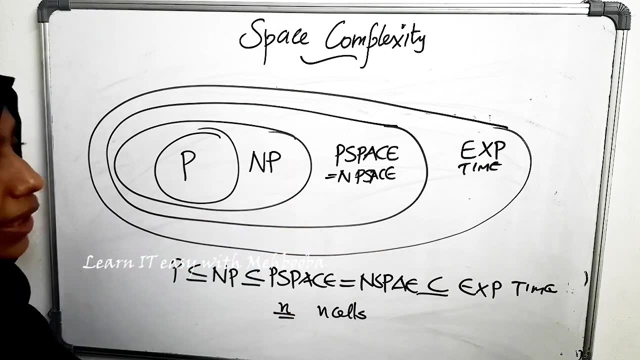 So that is why this P and NP classes are contained inside PSPACE and NP SPACE. Now, this reasoning will be given by Savage Theorem. why PSPACE is equal to NSPACE, that we will discuss in our next video. And next Next thing is exponential time. 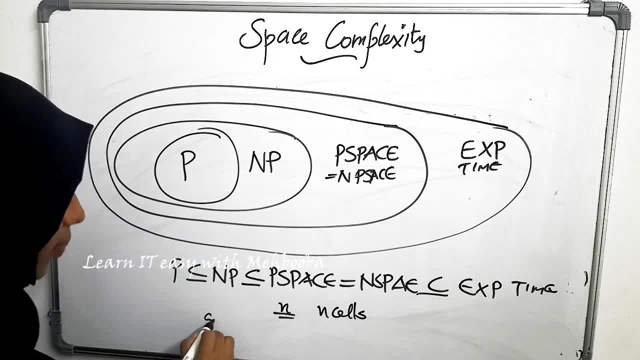 See for a non-deterministic Turing machine. if one branch is taking some SFN space, see if you are simulating that. you know that there will be two rays to SFN, different order of SFN, different configurations, right. 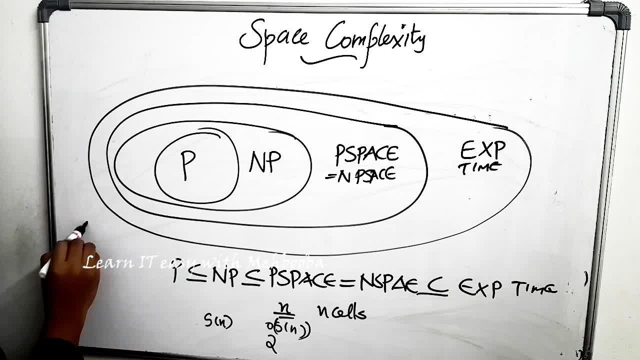 For example, if you are drawing, if you are converting an NFA into DFA, what happens? You are creating subset of every possible combinations of states For the DFA. that is, you will be having two rays to N states, states, power states made from this NFA for this particular DFA. 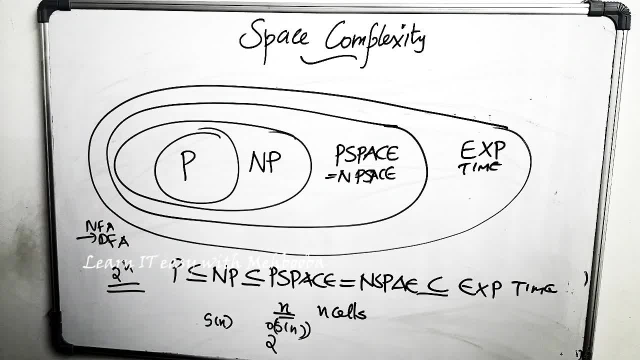 Similarly, if you want to simulate a non-deterministic Turing machine by deterministic one, you will be having two rays to order of SFN, different configurations possible, And they will in total will take SFN into two rays to SFN. yeah, computational space to perform this. 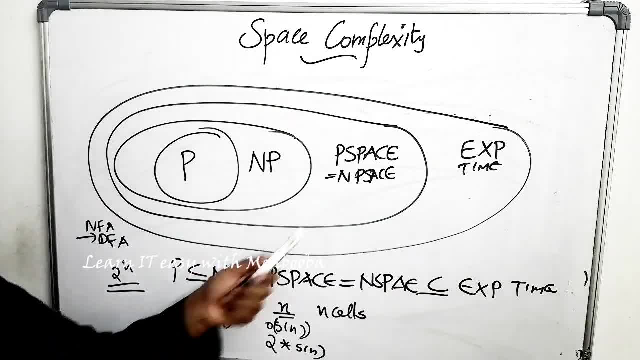 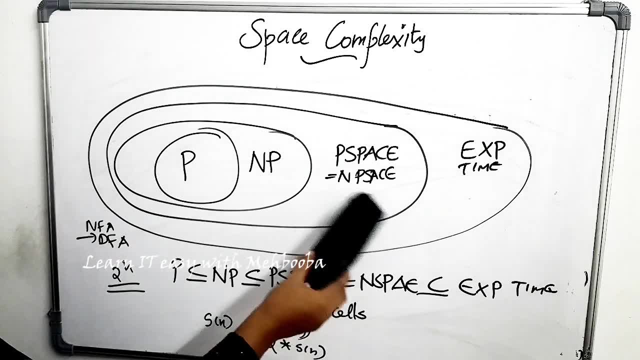 So explain: Exponential time takes most. I mean exponential time is higher than all of this, because to do this you will take even more than exponential time. So P space and N space comes inside the class exponential time. They are subset of the class exponential time.